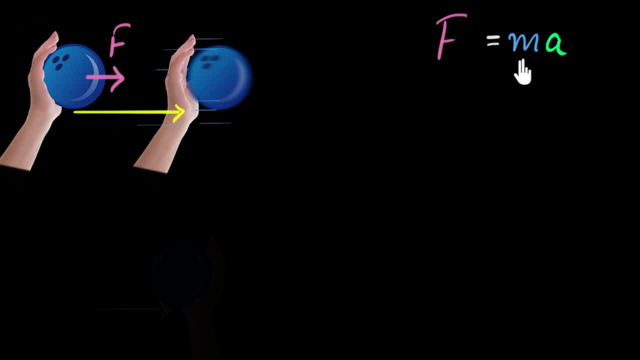 And this is in accordance to Newton's second law, which says F equals ma, which means force will accelerate a body. Of course, if there are more than one forces, then we have to calculate the net force, but we'll talk about that later. 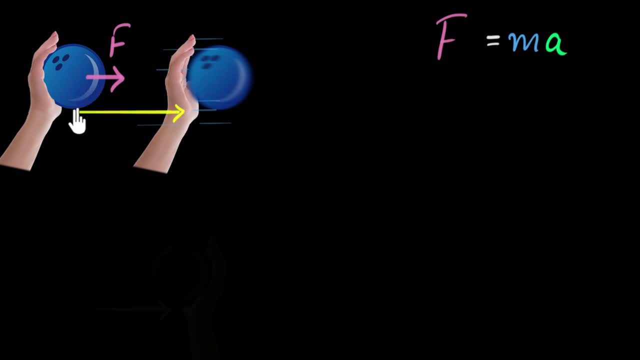 Let's consider only one force as of now. So you're putting a force and that accelerates the body. That's one way to think about it. Now let's think in terms of work done, You see, because you are pushing on it. 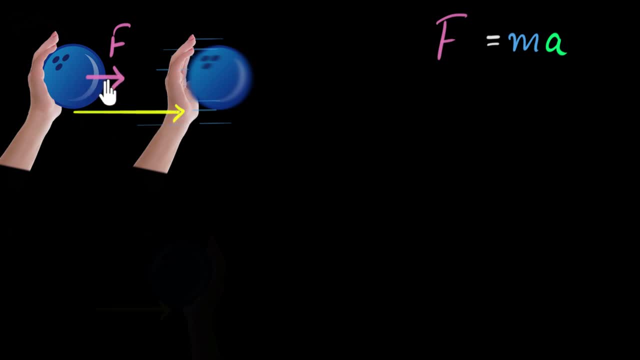 and you're displacing that body, you're doing work on that ball right And when you're doing work, look at what happened to the ball Initially. it had no speed, it was at rest, so it had no kinetic energy. 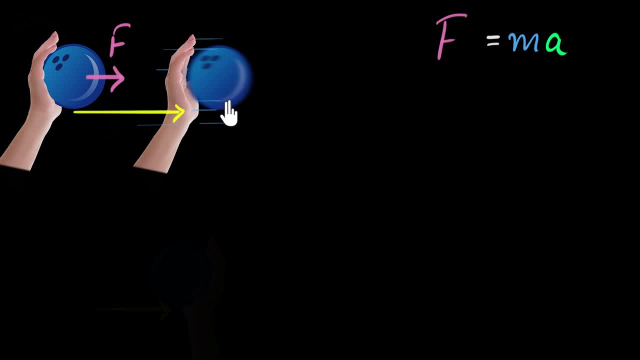 But then, after doing work, notice it has gained kinetic energy. So we can now say that by doing work we have added kinetic energy to our bowling ball. And so by doing work, whenever work is done on an object, kinetic energy gets added to that object. 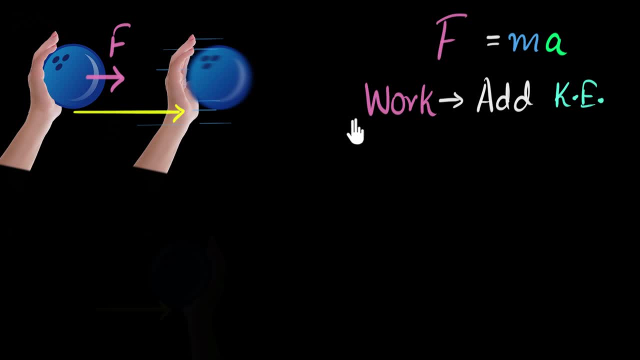 This is a new way of looking at the same situation. Now you can also do work and remove kinetic energy, if you want. For example, imagine a ball is thrown at you and you try to catch it. Now, when you try to catch a ball, like this again. 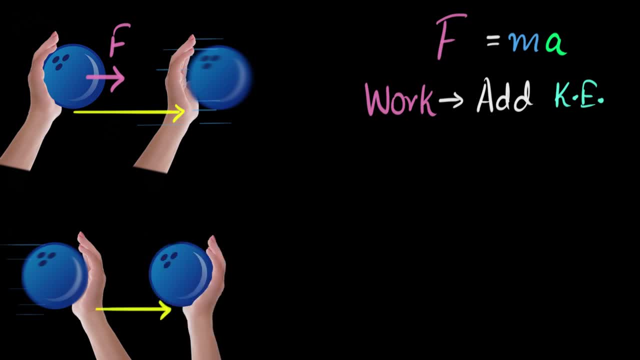 your hand will move back a little bit. Now think about what happened. When you try to catch that ball, your hand will start pushing it, but this time it pushes it in the opposite direction, And that's why it's slowing it down, right. 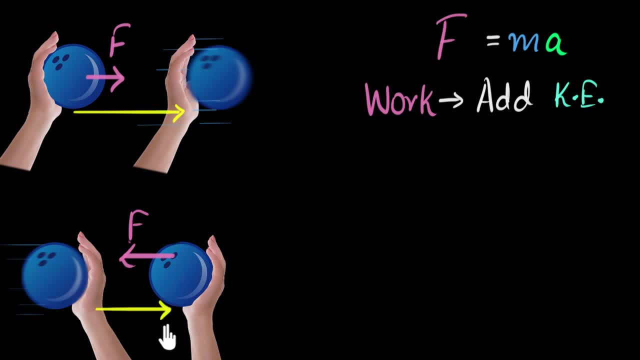 But now think about the work done, Because you're pushing it in the opposite direction to the displacement. work done is negative. And now, when you're doing negative work, look at what happened to the kinetic energy. The kinetic energy reduced. So we can now say when you do, 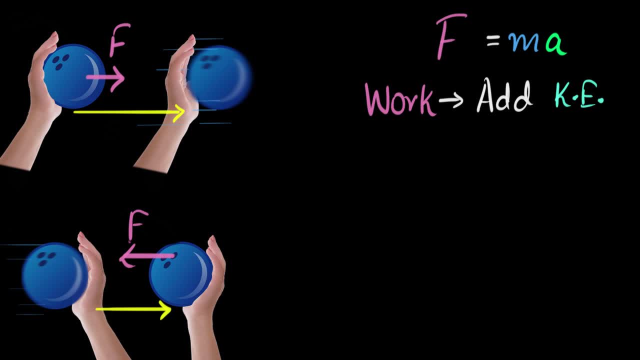 negative work, you are removing the kinetic energy from the body. So negative work removes kinetic energy from the body And this is, crudely speaking, what we call the work-energy theorem. It basically says: when you do work, you either add or remove the kinetic energy from the body. 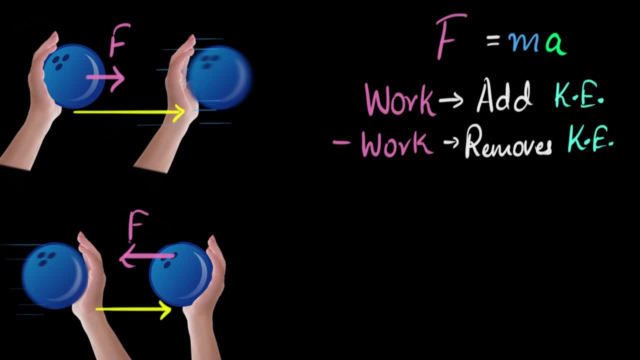 If you don't do work at all, then the kinetic energy will not change. Of course we'll derive the mathematical version a little bit later, but before we do that let's look at some more examples. Let's say, now you take that bowling ball. 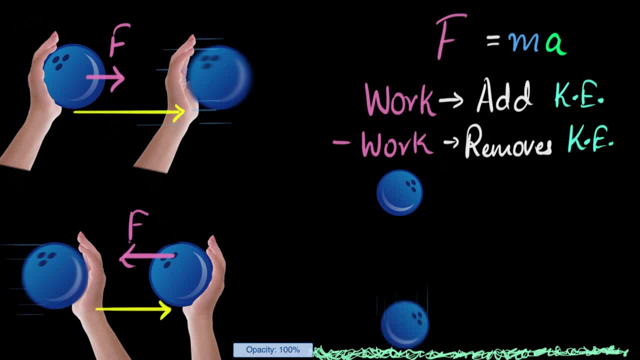 and you drop it from some height. Now, as it falls down, it's going to speed up Again. let's look at work. In this particular case, gravity is pushing down on that ball and the ball is moving in that same direction. 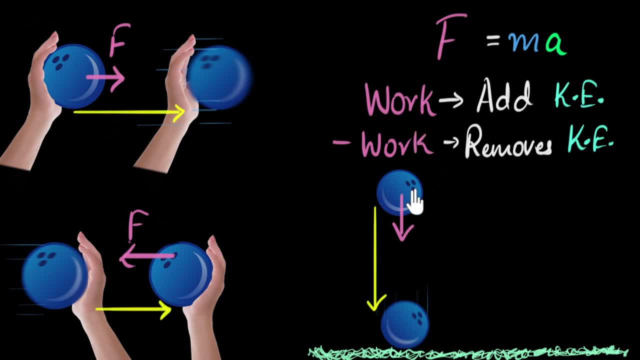 So gravity is doing positive work And because gravity is doing positive work, it's adding kinetic energy to that ball and that's why the ball is speeding up. Similarly, if you were to take that same ball now and throw it up, let's say you threw that ball up. 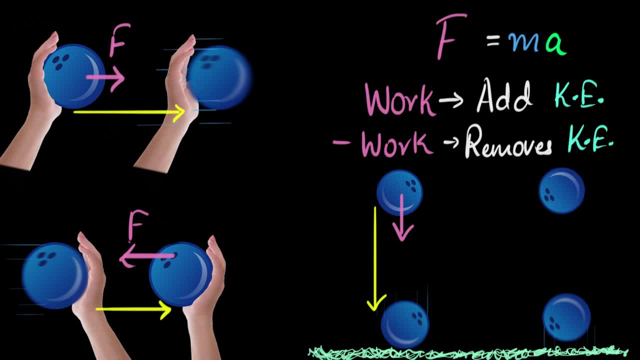 now, as that ball goes up, you might know it slows down Again. what's going on? Well, again, gravity is pushing down on that ball. Remember, gravity always puts a force downwards, but this time the ball is going in the opposite direction. 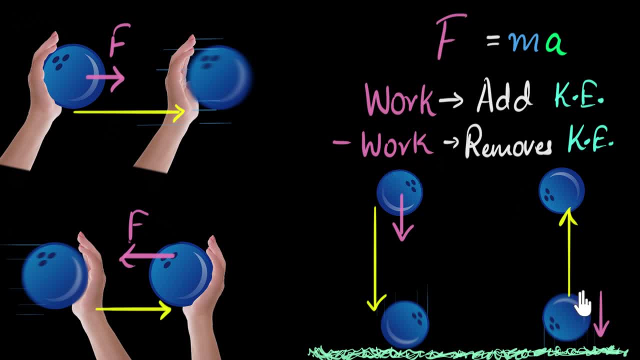 So gravity is doing negative work and, as a result, gravity is removing kinetic energy, and that's why the ball is going down, is slowing down. This is pretty cool, right, Thinking in terms of work and energy. Now things get even more interesting. 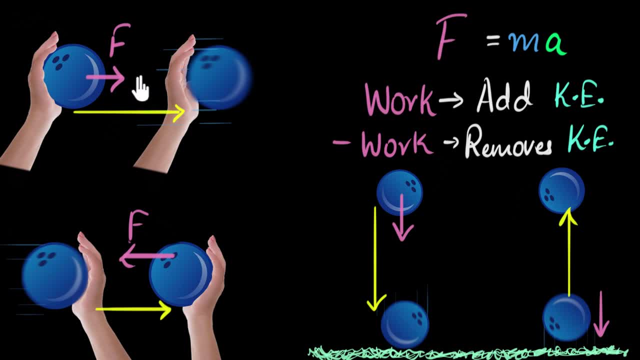 when there are more than one forces acting on the body. So, if there are more than one forces acting according to Newton's second law, we need to now calculate the net force Meaning. we have to add up all those forces. Well, of course, if the forces are in the same direction, 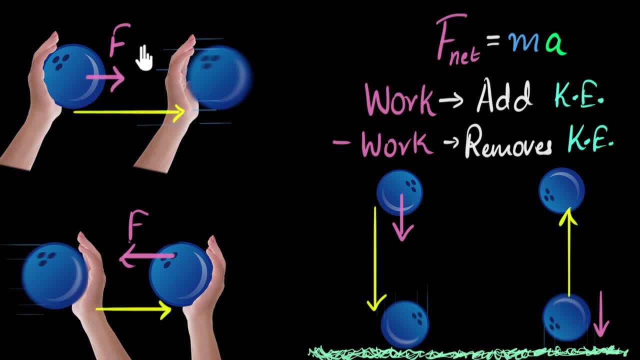 we add them. If they're in the opposite direction, we subtract them. But anyways, you calculate what the total force on that ball is and that will tell you what will be the acceleration of our body right Now. similarly, if there are more than one forces. 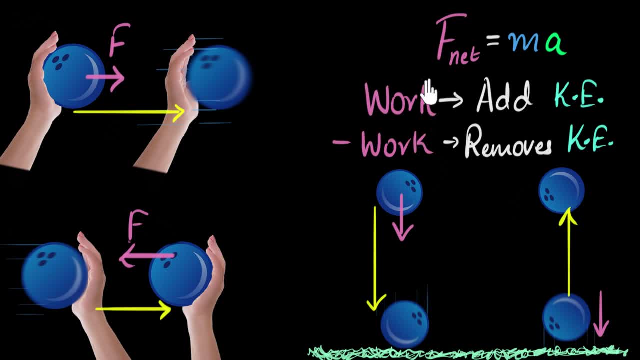 acting on the body. you calculate the total work done by all the forces and now that decides what happens to the kinetic energy. So if that total work done by all the forces becomes positive, kinetic energy will be increased and kinetic energy gets added. 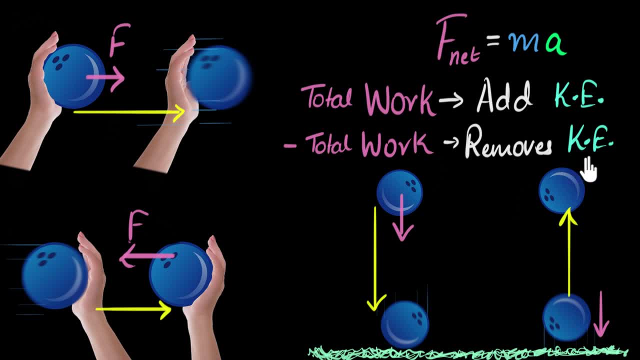 If that total work done ends up becoming negative, that means kinetic energy will be removed. And if the total work done is zero, which is totally possible, some forces can do positive work, others might do negative work, and we'll look at some example. 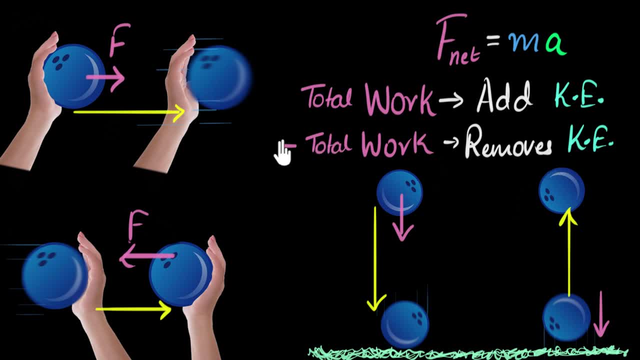 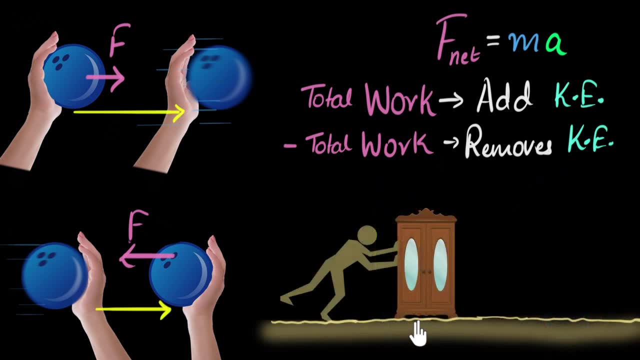 then the total work done can be zero. In that case kinetic energy will not change at all. Again, let's look at a couple of examples of that. Let's say there's a cupboard on a very rough floor, very heavy cupboard, and you want: 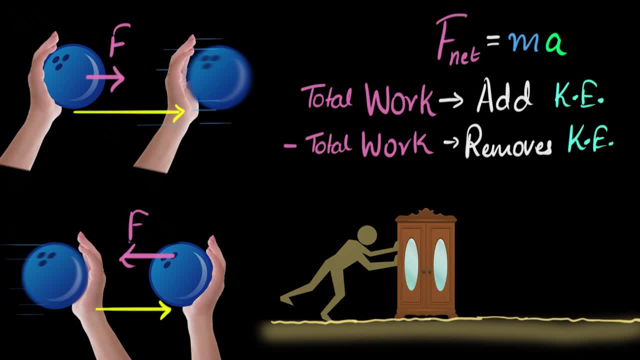 to move it. so you start pushing on it. Let's say, as you push on it, you slowly displace it from here to here. Now, after displacing, after you've pushed it, the cupboard is still at rest. So let's think about the kinetic energy. 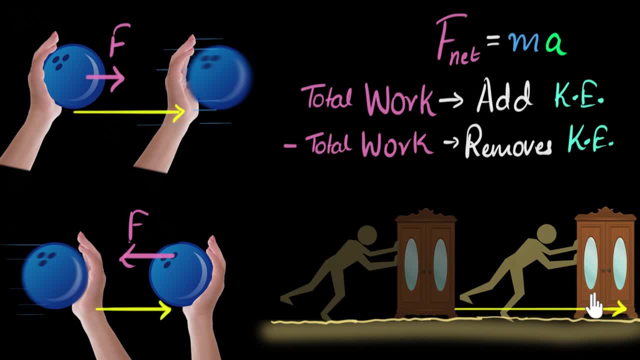 Initially the kinetic energy was zero. it was at rest After pushing. also the kinetic energy is zero. So the kinetic energy didn't change at all. So it was neither added nor removed. that means the total work done on this cupboard. 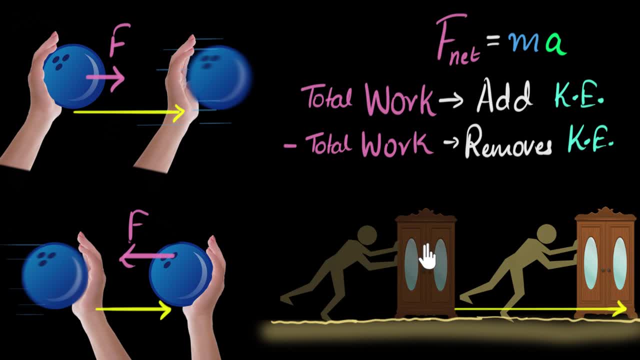 was zero. Why? Clearly, you pushed on it, you did work. then why is the work done zero? That's because there are more than one forces acting over here. So you are pushing on it and you are doing positive work. 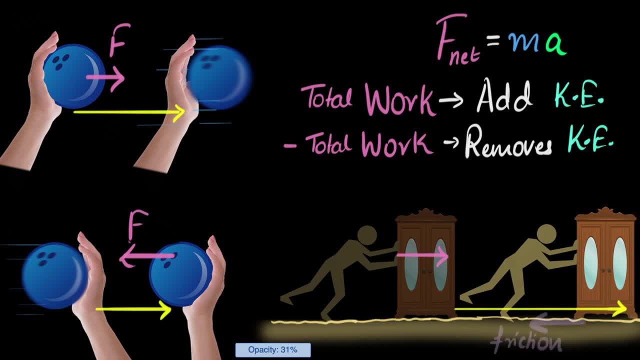 But because the floor is rough, friction is pushing on that cupboard in the opposite direction, doing negative work. So you are doing positive work, friction is doing negative work, so it just so happens that the two work done cancel out. 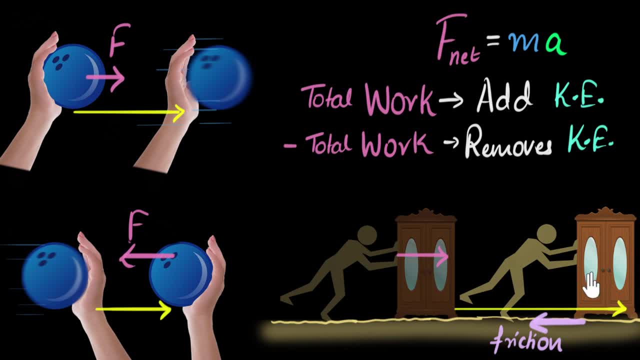 Total work done ends up becoming zero, And that's why the kinetic energy didn't change at all. Another way I like to think about this is when you're doing positive work, I like to think that you are adding kinetic energy to the cupboard, but at the same time, 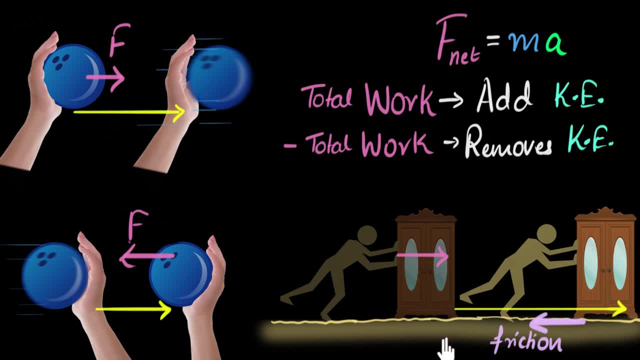 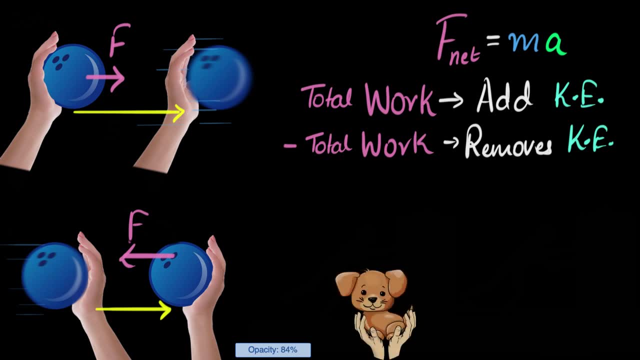 friction is removing that kinetic energy from the cupboard and that's why the kinetic energy didn't change at all. Okay, let's do one more, Say: I take this very cute puppy which is initially at rest. it's at rest right now. 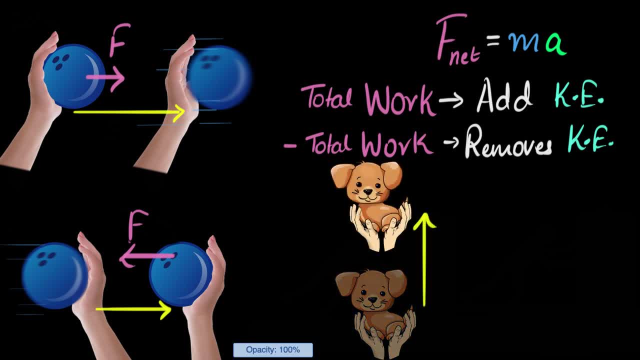 I push on it and I raise it up slowly and finally again it's at rest. So even here the kinetic energy did not change. That means the total work done on this puppy is zero. But why? Clearly I am pushing on it and I'm making it move. 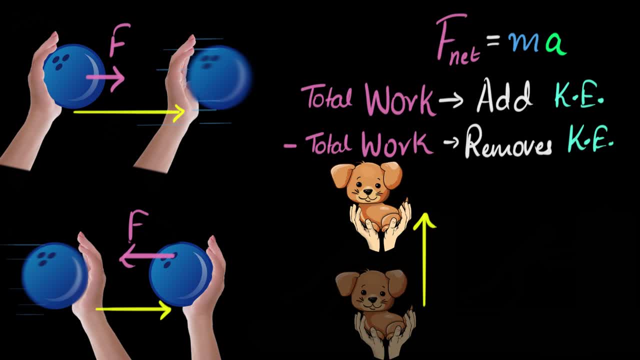 so why is the total work done? zero? Can you pause the video and think about this one? Well, again, I am pushing on it and I am doing positive work and I am trying to add kinetic energy to this puppy, But there's one more force acting on this puppy. 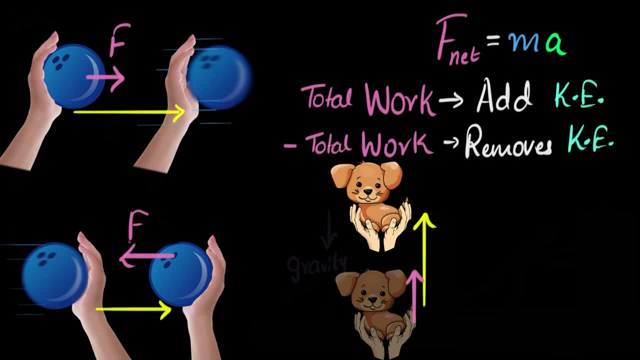 Which one Gravity. Gravity is pushing down on that puppy and, as a result, it's doing negative work because it's in the opposite direction of the displacement, and so gravity is removing kinetic energy from the puppy at the same time. So I'm trying to add kinetic energy. 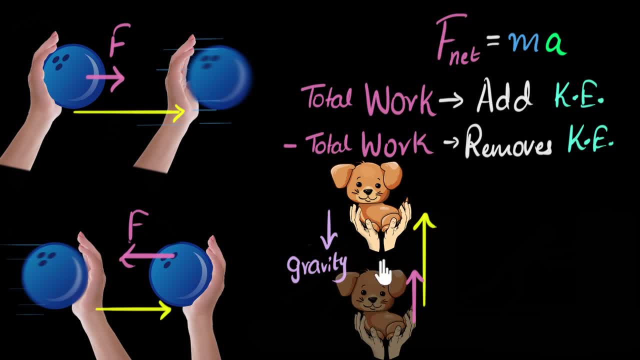 gravity is removing the kinetic energy, and that's why there is no change in the kinetic energy at all. So my positive work is canceled out by gravity's negative work, making the total work done zero. So now that we have some idea of the work-energy theorem, 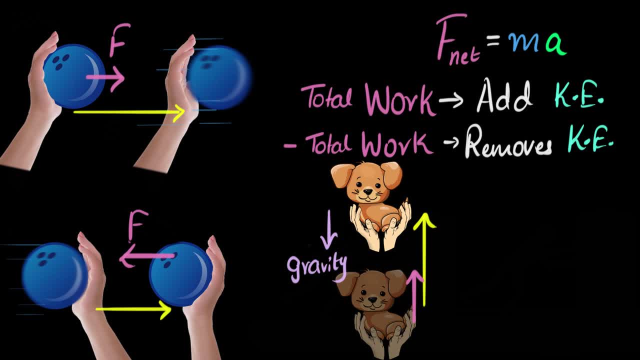 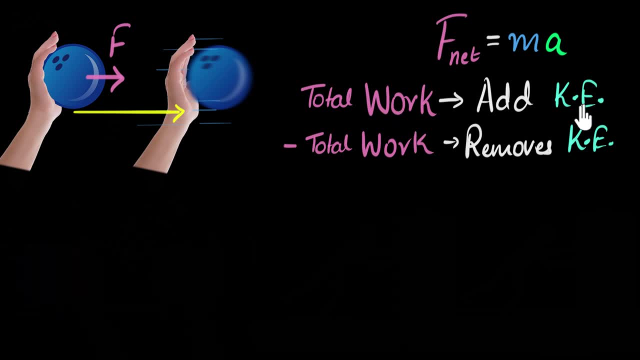 let's go ahead and derive the mathematical equation for it. This will be useful for problem solving. All right, so I need to connect work and kinetic energy, right? So again, let's start with just one force, If there's one force acting on the body, 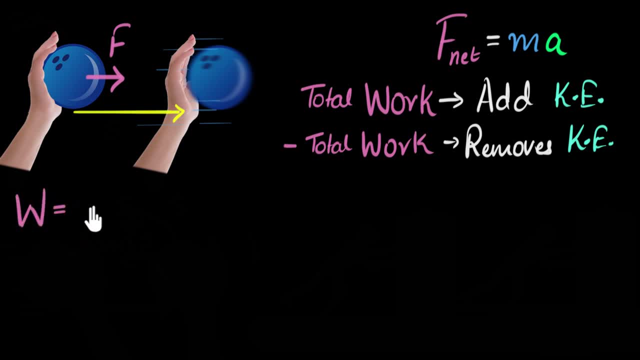 then the work done by that force. the work done would be the force multiplied by the displacement. Let's call the displacement as S. Okay, what do I do next? Well, I want to somehow bring velocities into the picture, because I want kinetic energy, right. 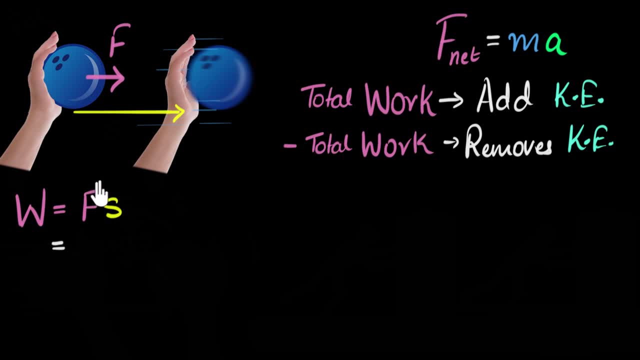 And I can do that by substituting F equals ma, because that's how acceleration comes, and then from acceleration I can bring velocities. So if I substitute F equals ma, so I'll get m times a times S, But I don't want acceleration. 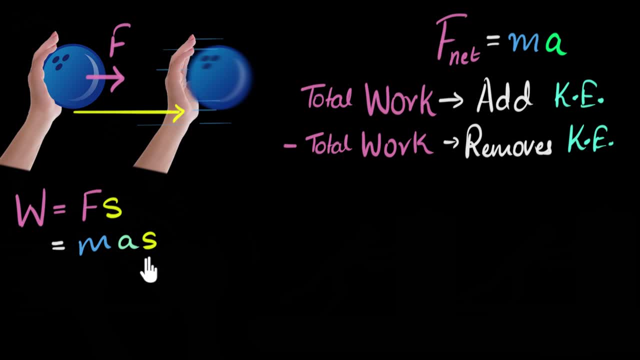 I don't want displacement, I want velocities. So can you think of a connection between acceleration, displacement and velocities? Initial velocity and final velocity. Yeah, go back to equations of motion. Think about this Great idea: to pause the video and see if you can remember an equation. 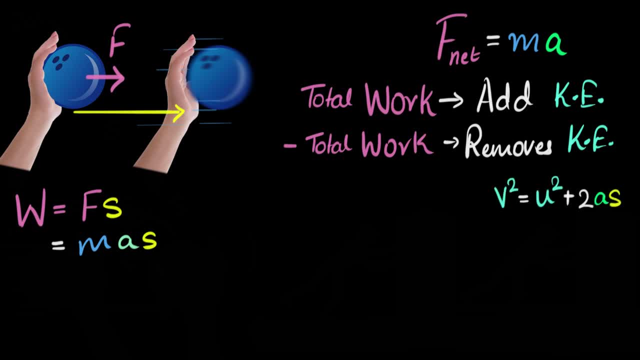 Well, there's an equation: v square equals u squared Z, plus two A S. This is perfect, because this will help us connect A S and write it in terms of V and U. So I want to get rid of A S, isn't it? 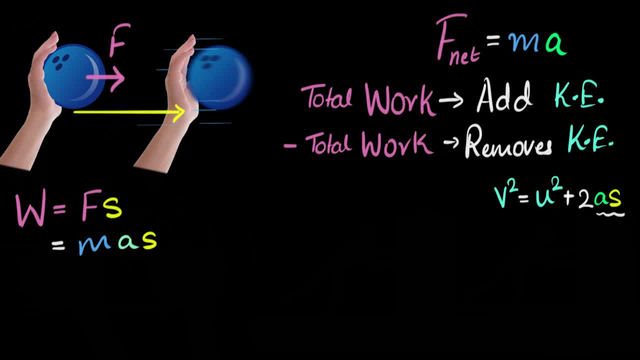 So let me isolate this on one side and put everything else on the other. So if I rearrange this, we'll get V squared minus U squared. divided by two, That equals A times S right. So now I can substitute that over here. 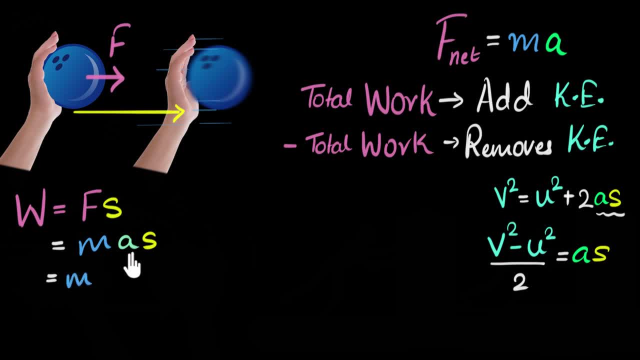 So that'll give me M times A. S is V squared minus U squared divided by two. Oops, let's use the same color: U squared divided by two. And now, if I open up that bracket, see what I end up with. Left-hand side is work and that equals. 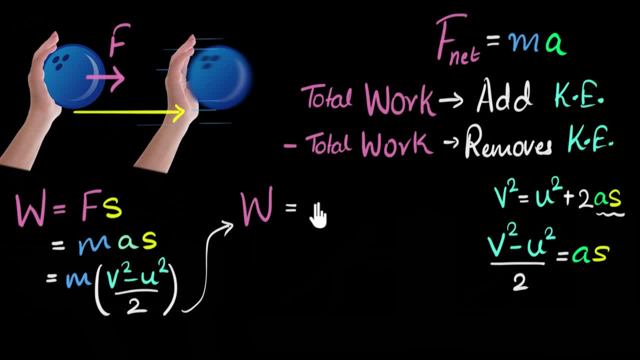 M V squared by two. what is M V squared by two? That's the kinetic energy, final kinetic energy. So we can call it as the final kinetic energy minus. you get M U squared by two. What is M U squared by two? That will be the kinetic energy initially. 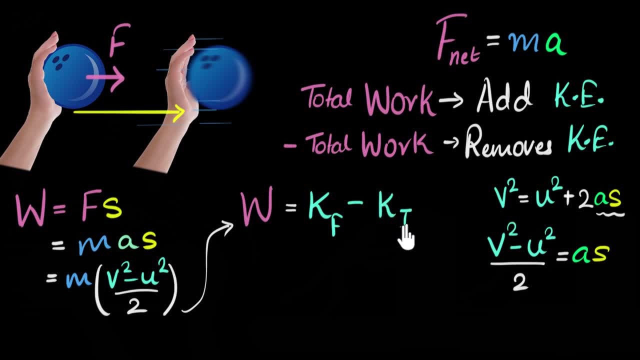 before I started pushing it. And this is the work energy theorem. mathematically It's saying the same thing that we discussed already. If you do positive work, notice the final kinetic energy will be more than initial. That means you're adding kinetic energy. 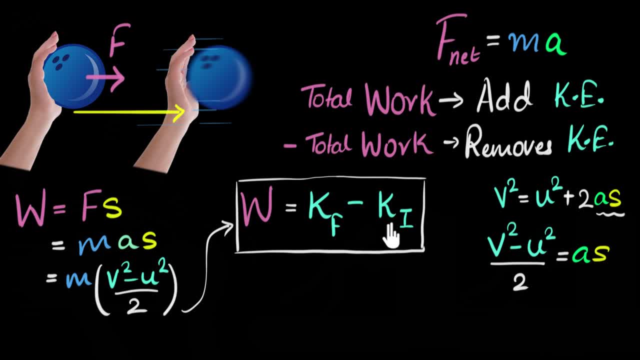 If you do negative work, you are removing kinetic energy. This equation is also telling that if you do 100 joules of work, as an example, then your kinetic energy will increase by 100 joules, So you will add 100 joules of kinetic energy. 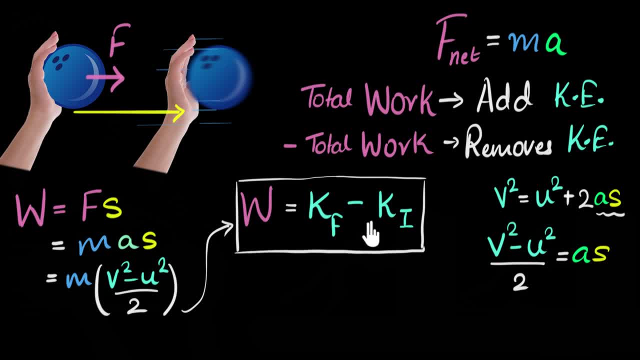 Similarly, if you do 100 joules of negative work, then you will remove 100 joules of kinetic energy. So you can kind of now see what work really represents. When you do work on a body, what happens to that body? 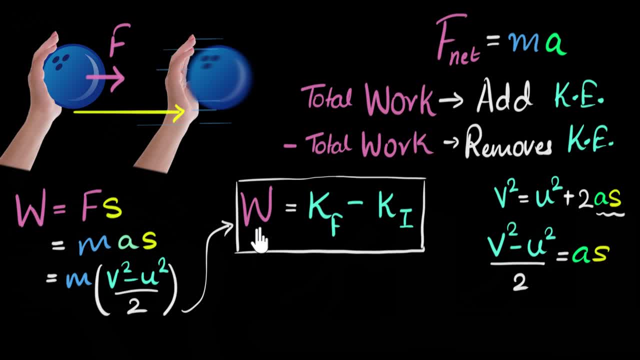 It's kinetic energy changes. So whatever work you do, that much kinetic energy gets added or removed. And again, if there are more than one forces acting on the body, what happens? Now you just have to calculate the work done by all the forces. 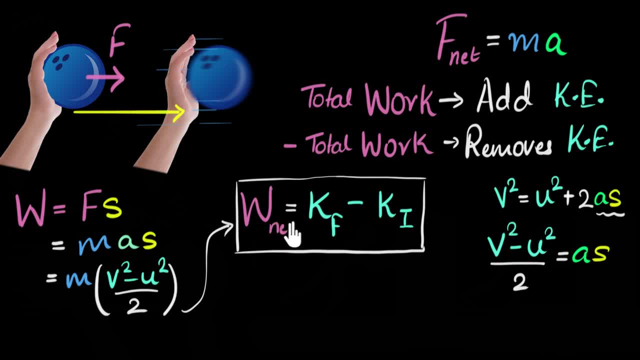 So we can say this will be the total work done, or we can say this is the net work done. So the total work done on a body will decide how much kinetic energy gets added or removed. And we will see in future videos that certain kinds of problems can be solved much faster.